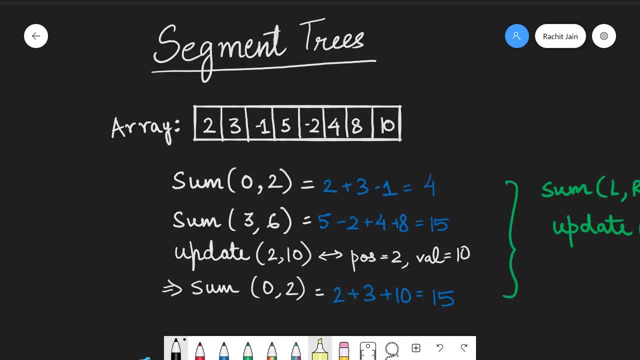 Hey guys, this is me, Rachit Jain, and welcome to yet another video. I know that a lot of people are always having second thoughts on segment trees. It's a really difficult topic for beginners, and what I want today is just go sit back and relax and watch this video. 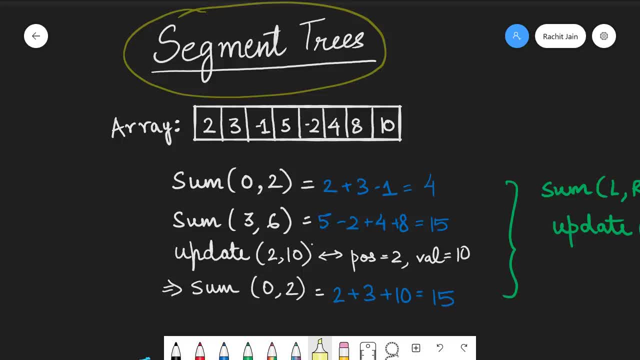 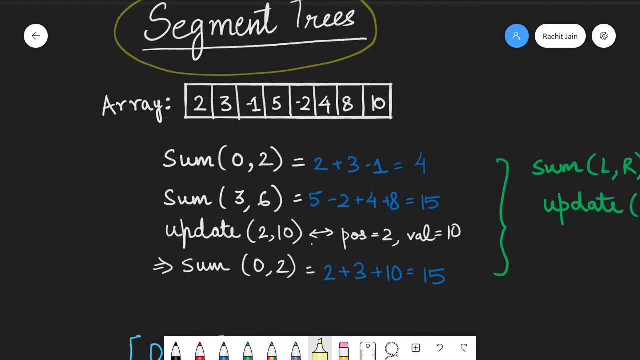 We will beautifully cover what segment trees are and how they are used in the world of competitive programming to answer queries faster and solve problems efficiently. So it's a data structure which is used on arrays to answer range queries easily in a faster way. So, for example, let's say we are having this array and we have to perform range queries In the range queries. 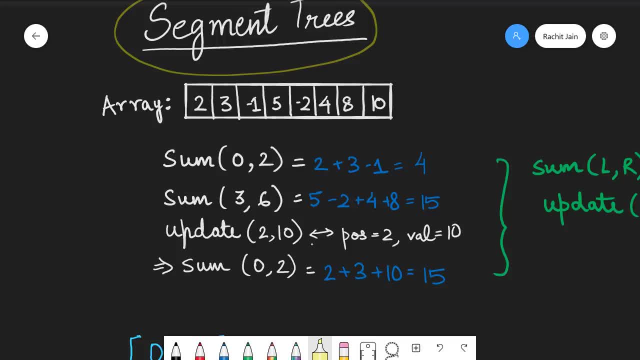 we are given a range or we are given a segment, and hence the name: segment trees. We are given segments of the arrays like 0 to 2, which is nothing but 0, 1, 2, from here to here, 3 to 6, which is 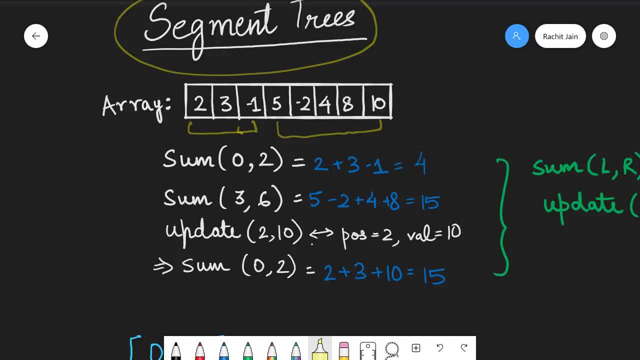 all the way up to here and we are asked the sum of that. So in this case, as you can see, sum 0- 2 is nothing but 2 plus 3 minus 1, which results in 4, and sum 3- 6, which is this one, it results in 15.. 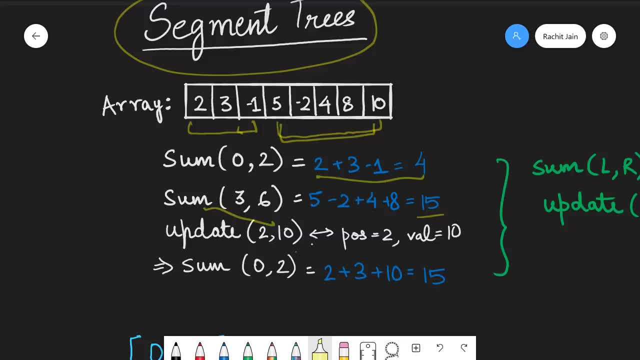 And then we also have queries wherein we are updating the elements of the array. For example, update 2 comma 10, which means this negative 1 now becomes positive 10.. That's what it means. and now when we do sum 0, 2 again, earlier it was giving us 4, now 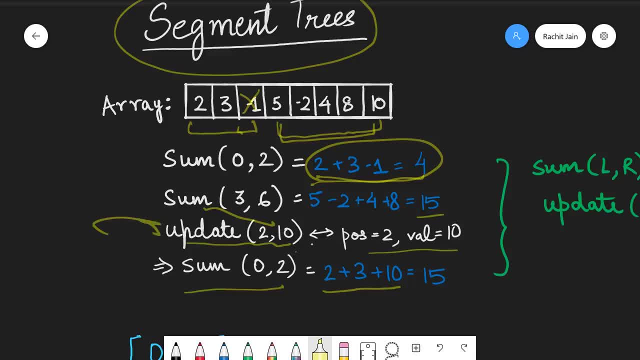 it's 2 plus 3 plus 10 because of this query, and then now the answer is 15.. These are the queries that segment trees allow us to answer in just log n time. So before jumping into log n and all those kind of things, right now, if we do brute force, like for example if we are given 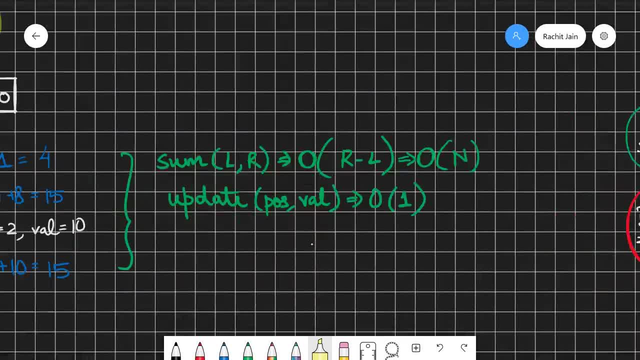 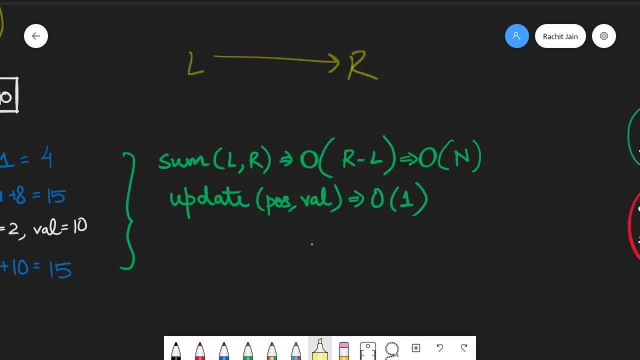 sum of L to R. So we will be performing a for loop and we will be going from L all the way up to R. So the time taken for that will be order of R minus L and in the worst case it can go order n. 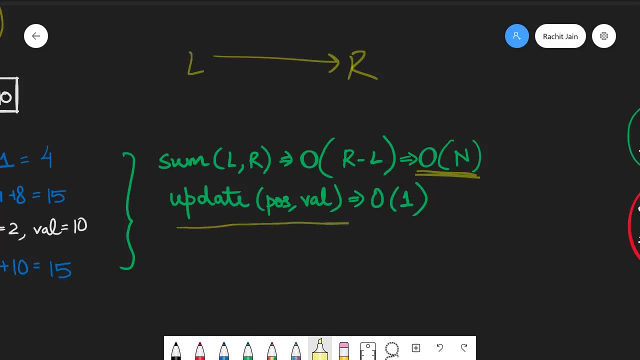 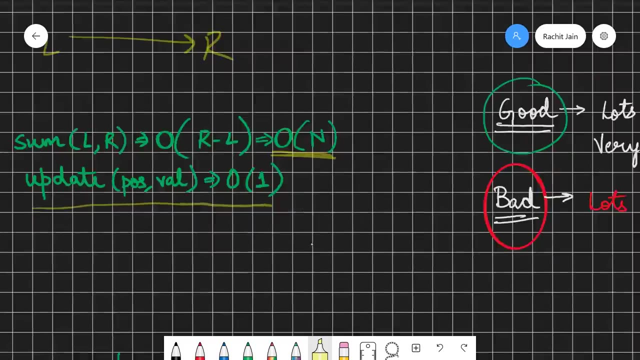 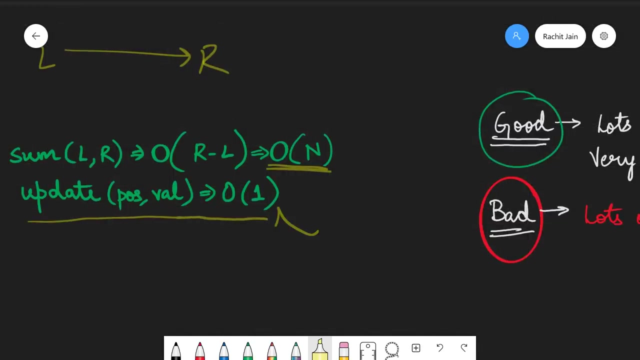 And for the update query, which is we just need to update the value for the array and that takes order one time. So this is what the brute force solution is suggesting. So what is the good thing about this brute force solution? The good thing is that if you are having lots of updates- okay, lots of updates, since it's handling updates with really very fast- 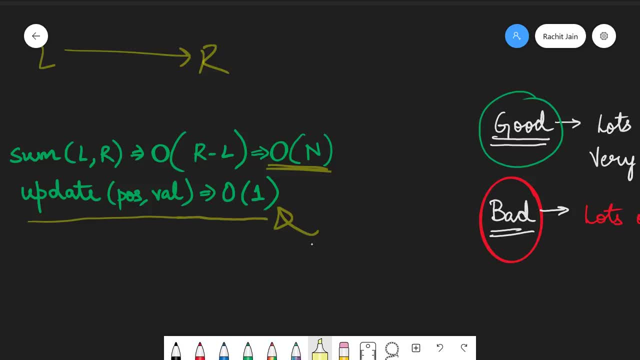 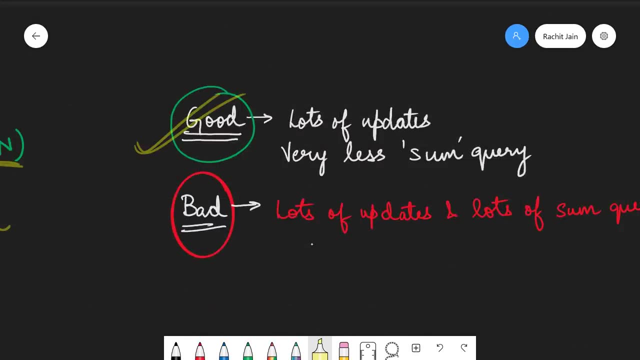 So in the scenario if you are having lots of updates and very few some queries, this, the brute force solution is very good. So that's what I have written over here. So for lots of updates and very less some query, this brute force solution is good. 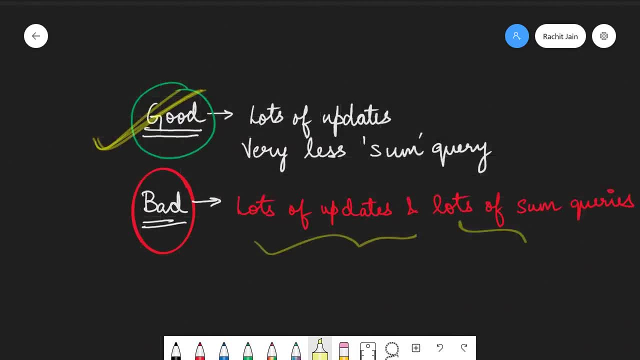 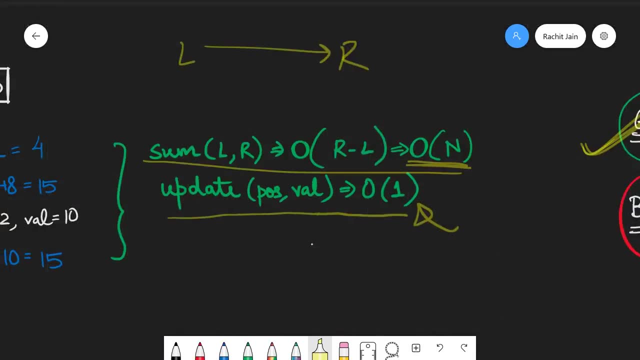 But it's bad when we have lots of updates and lots of some queries because each query can take order n time, as, as you can see over here, the worst case can go up to order n, where in we are going element by element and adding that in our sum value and finally printing that up. 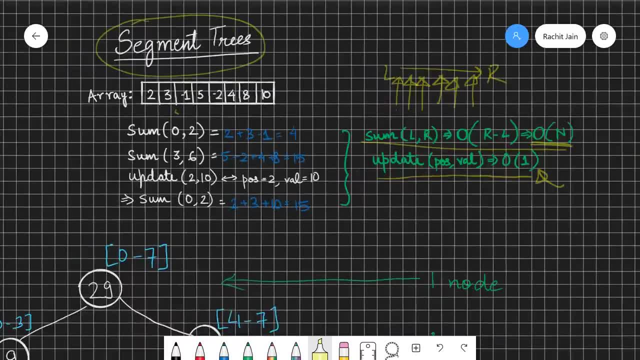 So how segment trees can help us over here. Let's see that. So for this array- 2, 3 minus 1, 5 minus 2, 4, 8, 10 that we are having over here- Let's construct the segment tree for that and have a look. 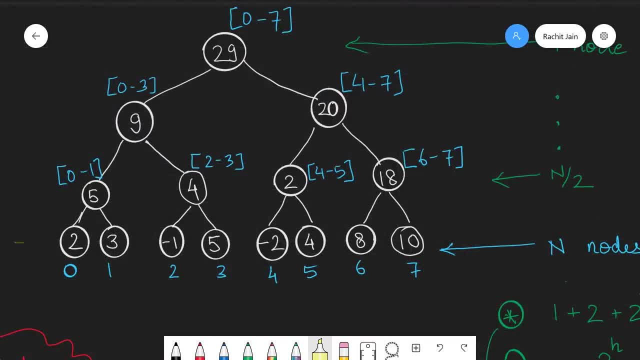 So, as you can see, the complete array that we were having is at the leaf nodes for this. This is the segment tree. I will quickly explain what I have written in this Blue nodes, or the blue segments that you are seeing like over here and here We will come to that. 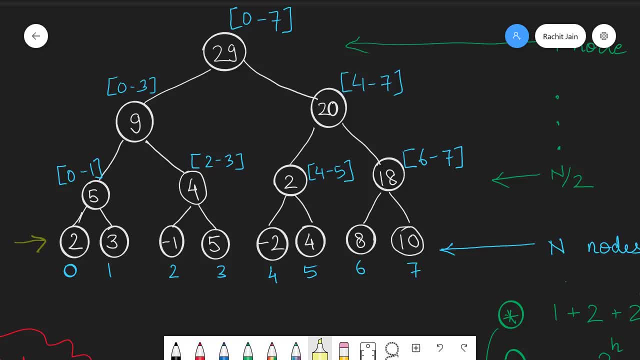 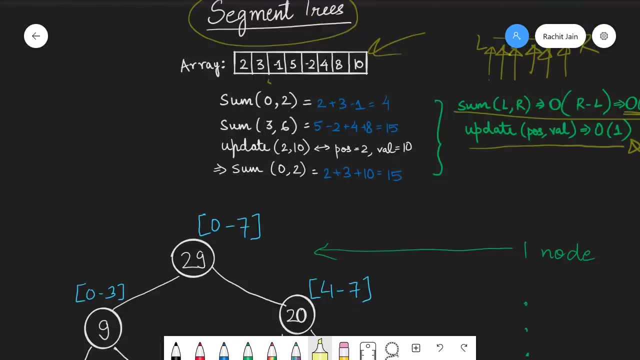 But first thing that I want you to notice is that the array that we were having was of size, I think, 8, if you can go back. Yeah, we were having 8 elements over here and the thing that we can see over here is the leaf nodes are nothing but exactly the array elements. 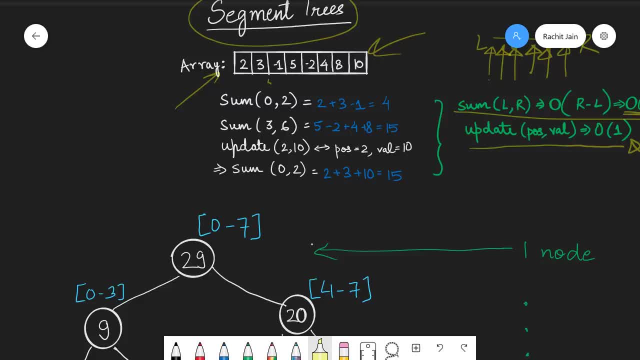 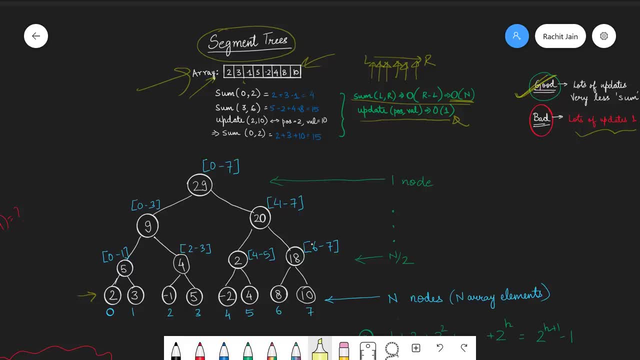 So, as you can see, 2, 3 minus 1, 5 minus 2, 4, 8 and 10, and if I zoom out a bit, I think you can see that clearly for yourself. So, as you can see over here, Compare this array right over here with the leaf nodes. 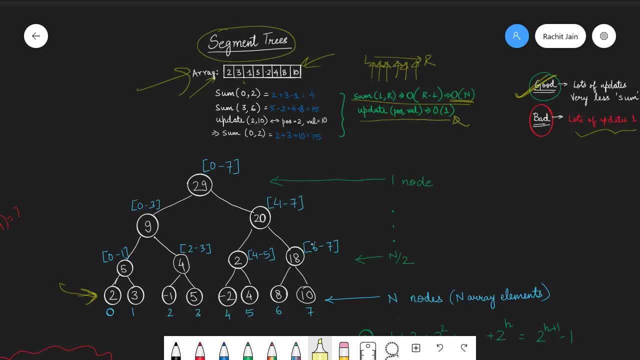 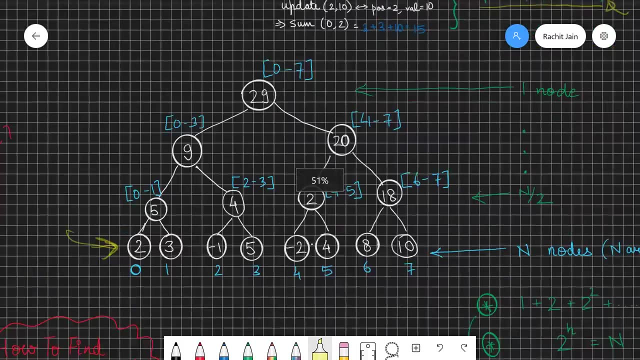 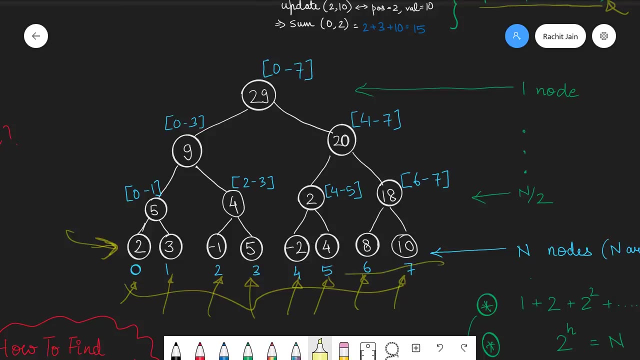 It's exactly the same: 2, 3 negative, 1, 5 negative, 2, 4, 8 and 10.. Alright, so what is this now? Let's let's focus on that now. Okay, I will zoom in back. Okay, so the leaf nodes are nothing but the original array elements. as you can see, 0, 1, 2, 3, 4, 5, 6, 7 are nothing but these. 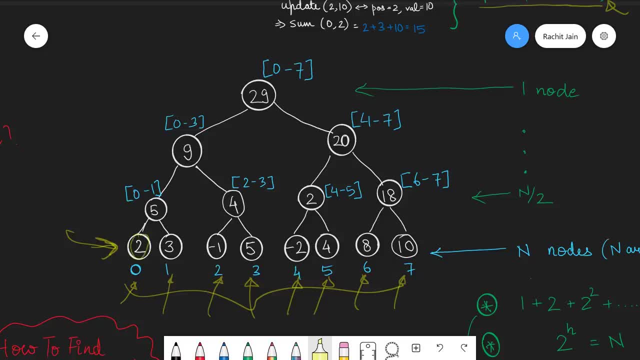 These are nothing but the indices and the leaf node values. as you can see, 2, 3 negative, 1.. These are the values of the array. Now the interesting thing is, We are creating these nodes in this layer that you can see. these are nothing but the sum of the leaf nodes. 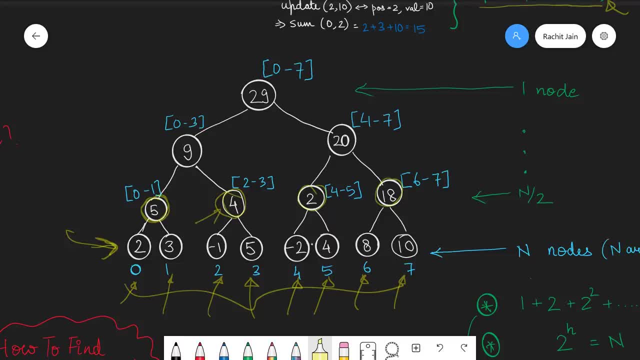 So 5 is the sum of 2 and 3. this right over here is the sum of negative 1 and 5.. This guy over here is the sum of negative 2 and 4, and this guy over here is the sum of 8 and 10.. 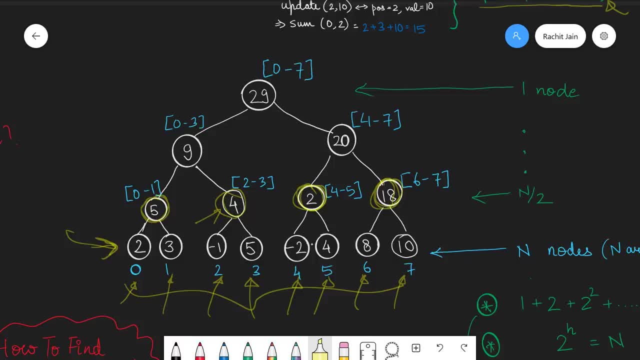 So what does this mean? So this node, which is having the value 5, is nothing but storing the sum of the elements from the range 0 to 1.. This is storing the sum of elements from the range 2 to 3, as you can see right over here. 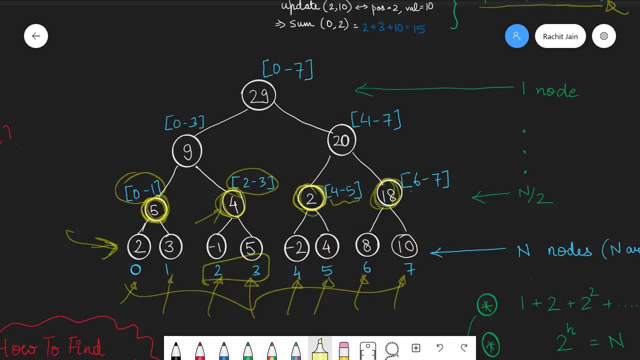 This is storing the sum of elements in the range 4 to 5, and this is storing the sum of elements in the range 6 to 7.. So what can we do next now? Now we can build this layer that we are having over here with value 9, which is nothing but the sum of this and this. 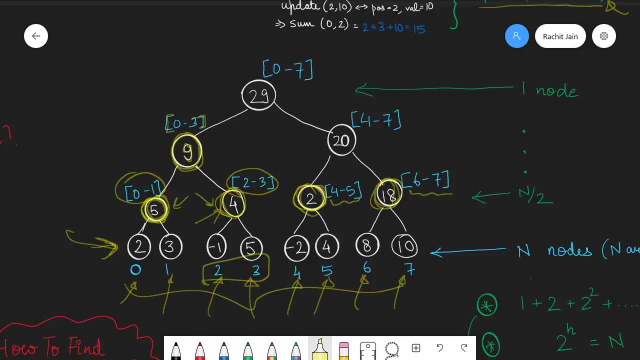 And this is storing the sum of elements from 0 to 3, and this is 20 over here. This guy is storing the sum from 4 to 7 and then, finally, the root node is storing the sum of complete array. 0 to 7 is the range for that and the value is right over here. So is this useful? 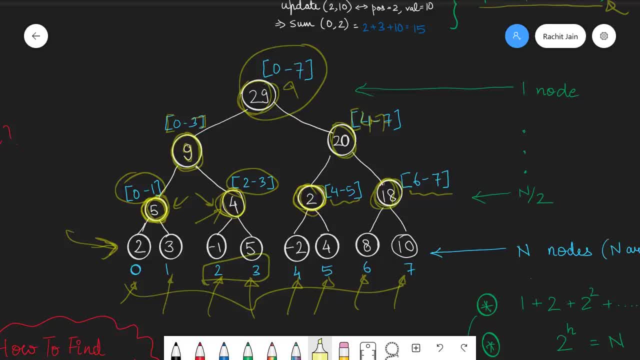 Do you think this is useful? Of course this is useful. Now we have a couple of nodes which are storing the sum of some segment of the array, As you can see this: 4 to 7,, 6 to 7,, 4 to 5,, 2 to 3.. 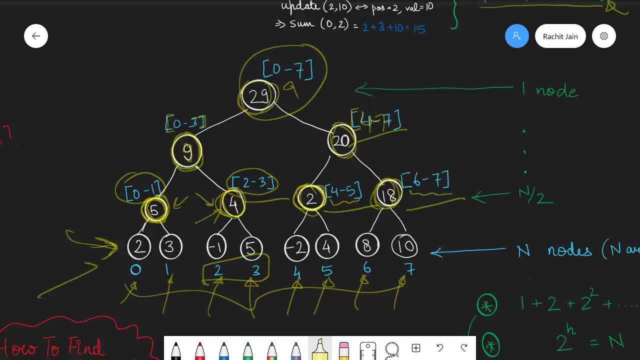 These are segments in the original array. Thus the leaf nodes are nothing but segments of size 1, and as we go one level up, the segment size increases by 2.. As you can see, all the values over here are are nothing but sums of segment size 2.. Here the segment size becomes 4 and here the segment size 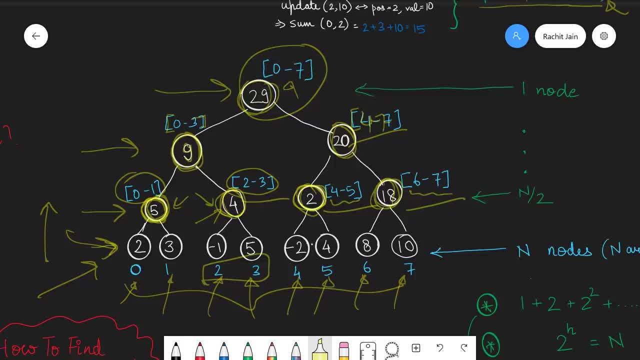 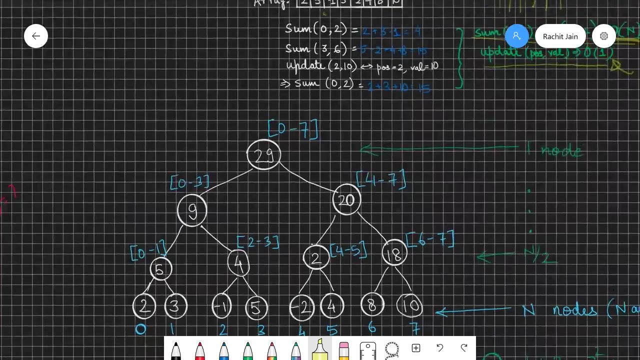 becomes 8.. So this is what segment tree looks like: Nothing but storing sums of various segments of the array, and this is something which we are going to leverage to answer queries really, really fast. So let's see how's that happening now. So now let's say, going back to the original queries, that 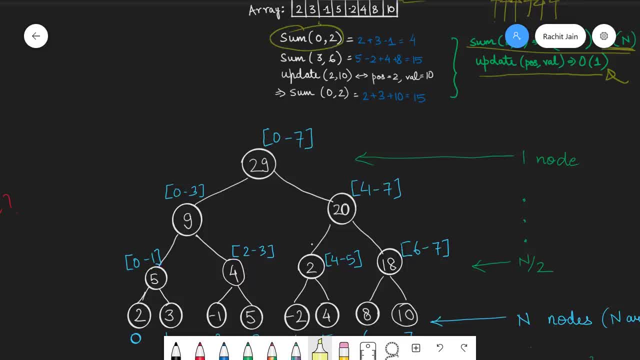 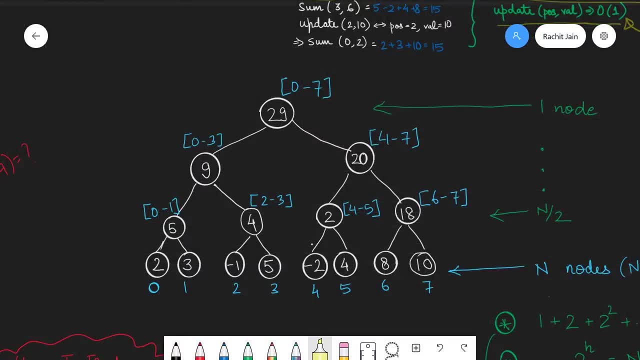 we were having. Now we are asked the sum 0 to 2, which is right over here, and we know the answer for that is 4.. Now let's use the segment tree to find this particular answer. Alright, so to find the sum 0 to 2, what I can use is: I can use this guy over here. It's giving me the sum of 0 to 1. 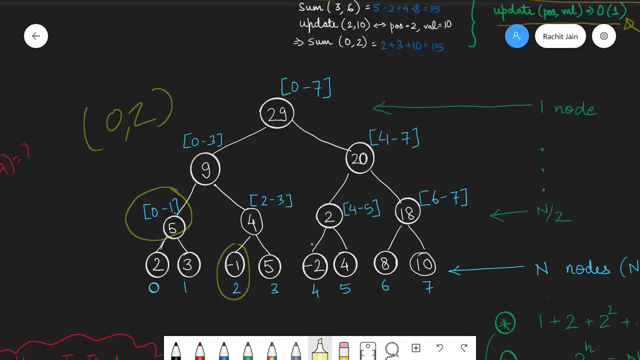 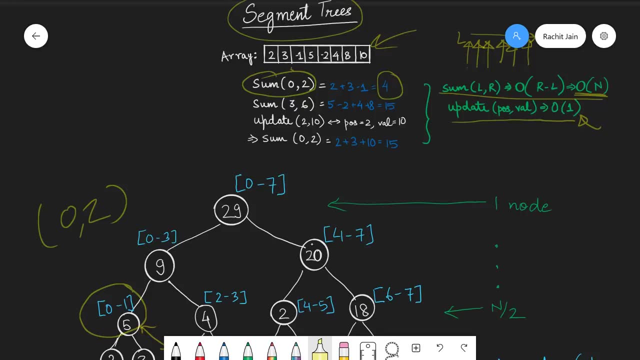 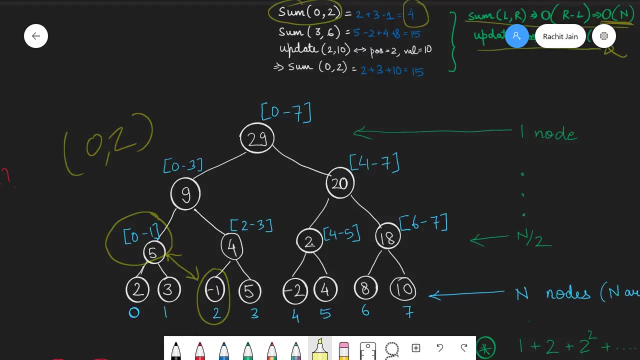 and now I just need the sum of the second element which I can take from here. So I will just do the addition of 5 and negative 1, which gives me 4, and that is exactly what we are having over here. So to take the sum of 3 nodes, we just used 2 nodes over here. Of course that's not huge. 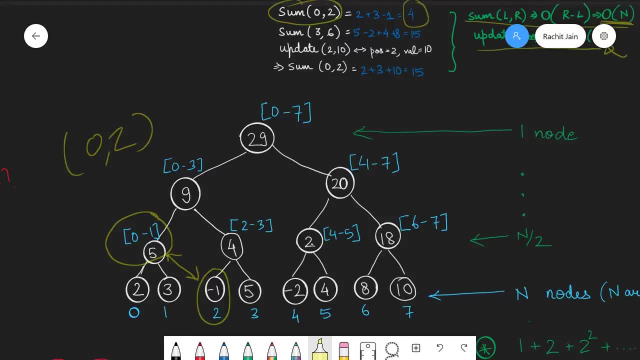 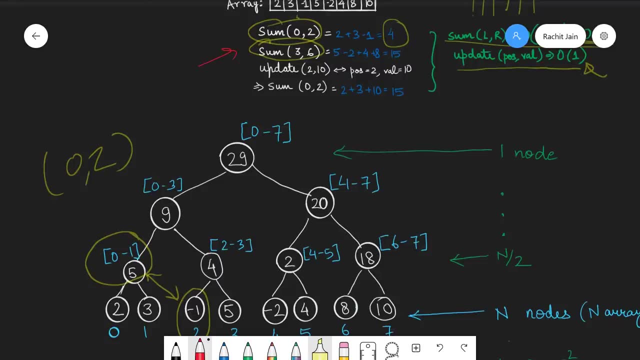 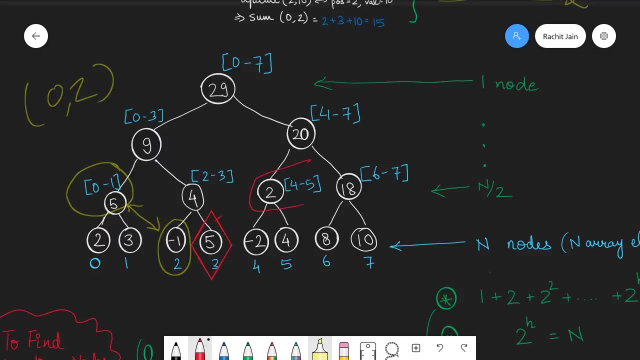 difference. as you can see right over here, That's not a huge difference for now, but when the ranges become high it really becomes efficient, and we'll come and we'll see that in a bit. So now let's try answering the query sum 3 to 6.. That can be found from a segment tree by using the node this, then 4. 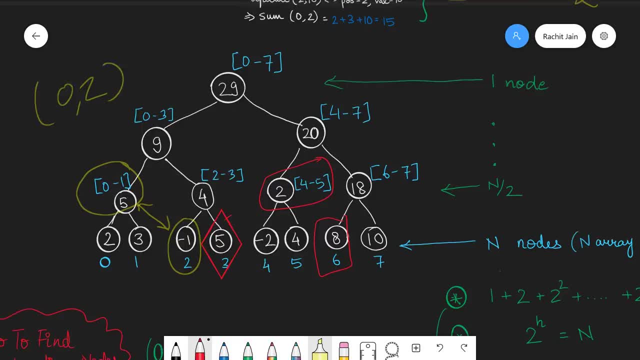 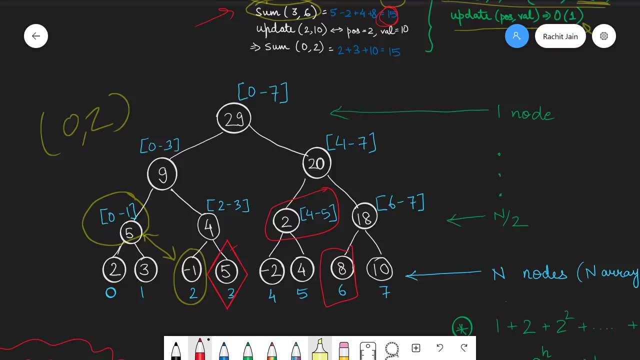 to 5 right over here and 6 node over here. So the sum now becomes 5 plus 2 plus 8, which is nothing but 15 and going back, as you can see, we are having 15.. What I want to stress right now is that 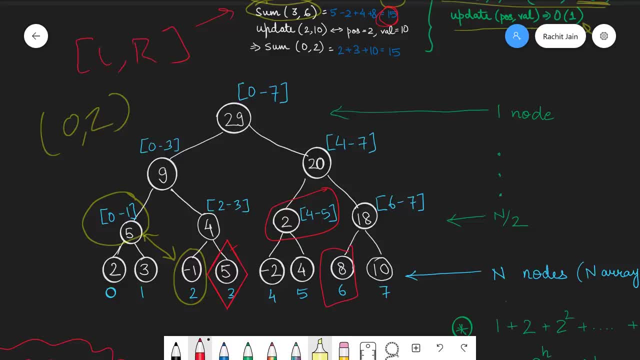 to get the sum of any range L to R. we can pick up some nodes or we can select some nodes from the segment tree that we are having over here and they will give us the answer for the sum of the elements from the range L to R. Why? Because we already have pre-computed the sum of various segments. 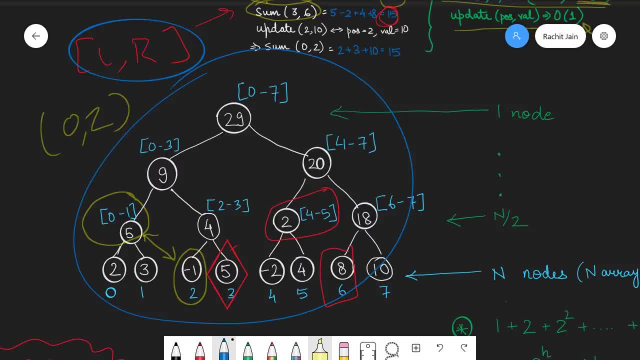 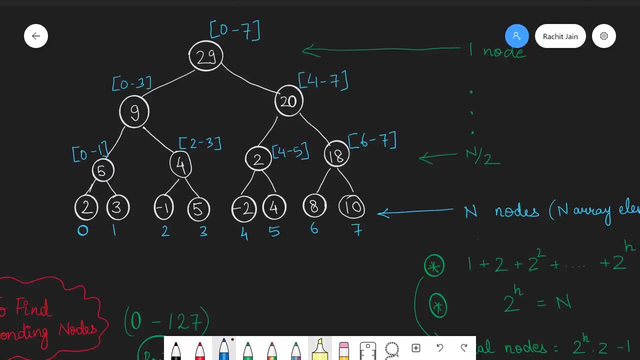 and the segment L to R can be broken down using those segments and we can sum the values of all these to get the answer for this. Another thing that I want to highlight over here is that so if the array size is n, we will be having around n leaf nodes. 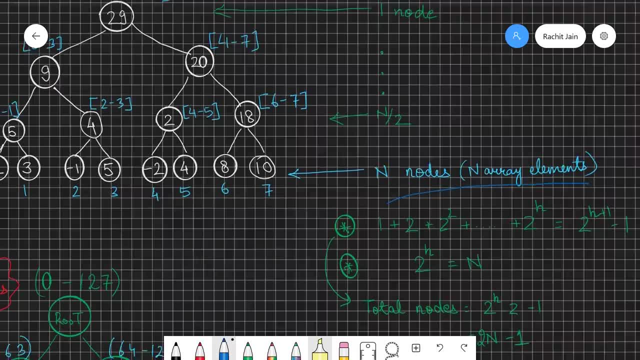 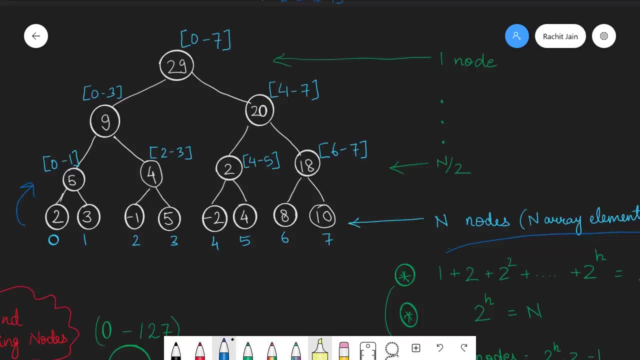 corresponding to the n array elements. and, as you can see, it's a perfect tree in the sense that the number of nodes in one level up becomes exactly half, just because of the way this tree has been constructed. like way here were eight nodes, here are four, and then two and then one. so the number 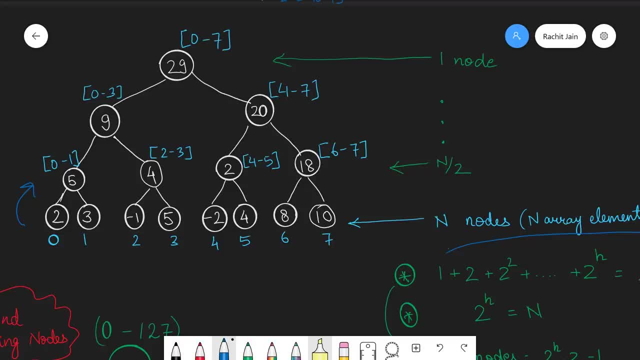 of nodes is decreasing by half, so the height of the tree becomes log n, because there are n nodes over here, and each time you are reducing the number of nodes by half, so eventually the height of this tree will be log n- Awesome. Another thing that I want to highlight over here is: 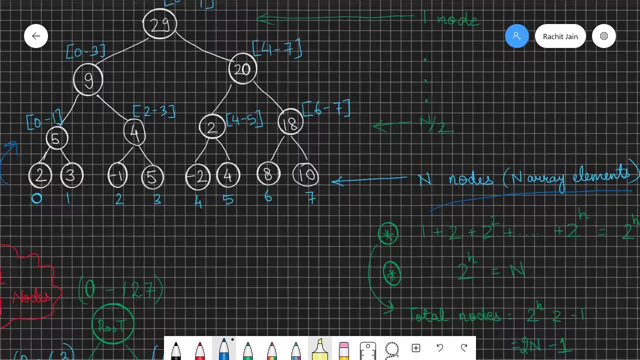 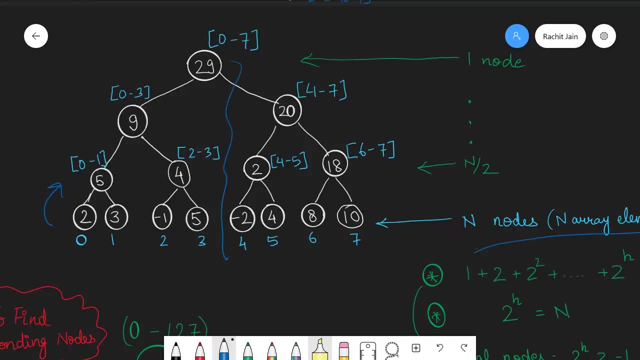 that? what are the total number of nodes in this? So okay, now let's say the height of this tree is h. so, as you can see, at the root we have one node, in the next level we have two nodes, in the next we will have four, and so on, and then, finally, if we have the height is h in the last level we will be having. 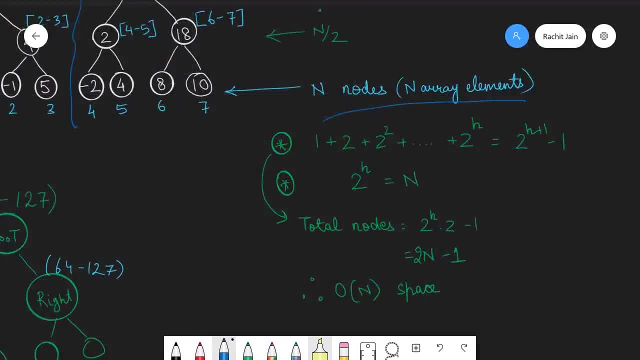 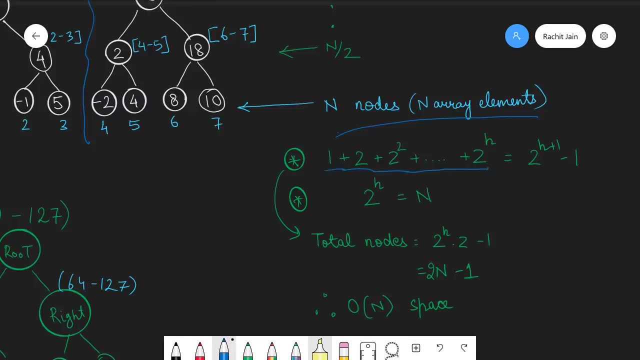 two to the power h nodes. So what we can say is that the total number of nodes in the segment tree is nothing but one plus two plus two square, and so on, up to two to the power h. This is a simple GP formula which you will evaluate. 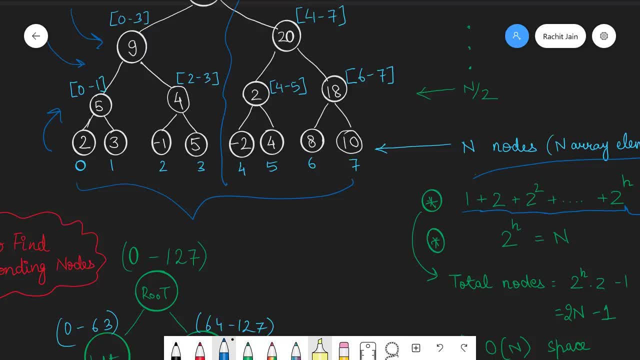 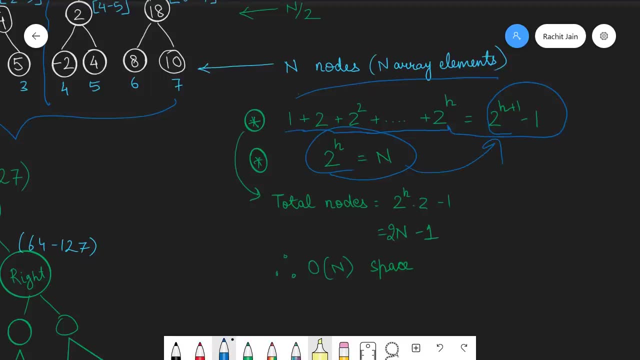 out to this. so the number of leaf nodes is n, and that's also equal to two to the power h, because h is the height of the tree. So now, substituting this in this equation, what we can get is that the total number of nodes is nothing but two, n minus one. so that space complexity for segment tree construction. 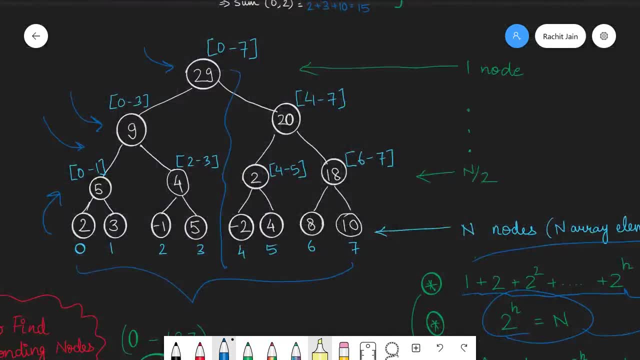 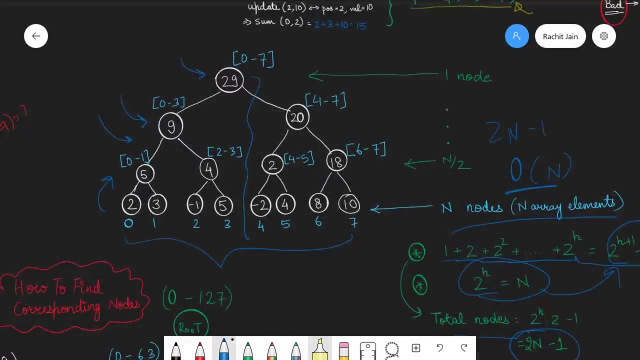 is just order n. Okay. so we were having n nodes in the leaf and we have constructed this tree, but the total number of nodes were two n minus one, and two n minus one is nothing but order n. okay, so the space complexity is also pretty good, Awesome. Now how are we handling this update query? that's something which we have. 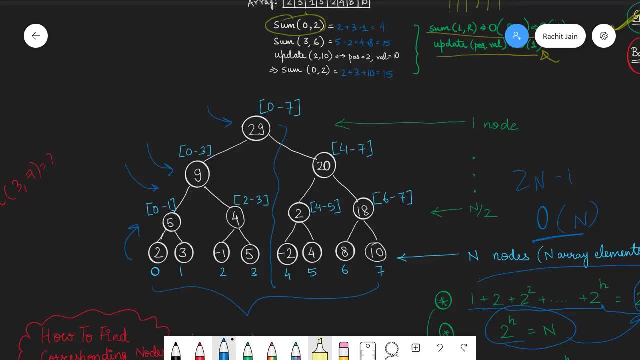 missed right now, so let's handle that as well. So now, when we get a query like update 2 comma 10, what do we do So? when we are getting some query like update 2 comma 10, what do we do? So when we are? 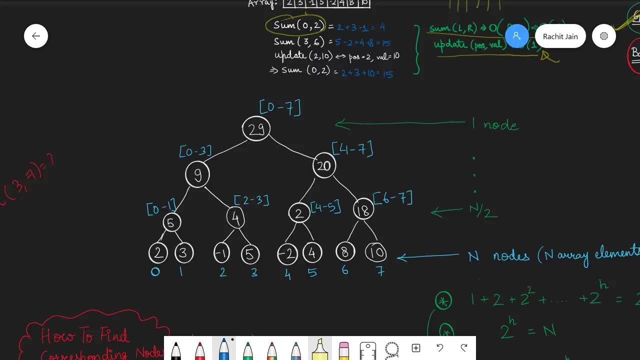 getting some query like update 2 comma 10. what do we do? So when we are getting some query like update 2 comma 10, the interesting thing that you will notice is that only this value is changing right. and since this value is changing, this value will also change. and since this value is changing this, 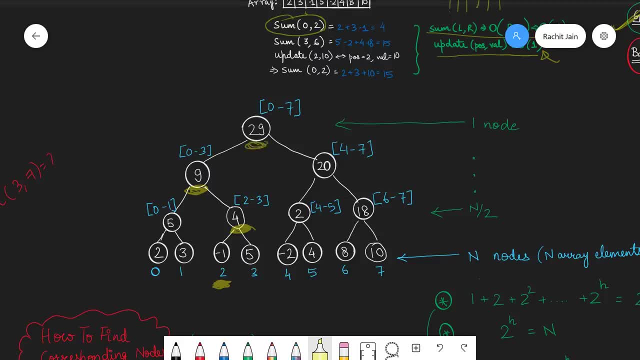 value will also change and since this is, it will change. this will also change. So in the complete tree, we only have a particular set of nodes which are changing, and that's nothing but the nodes which are falling in the path, from all the way from the root to the leaf node which is changing. So when 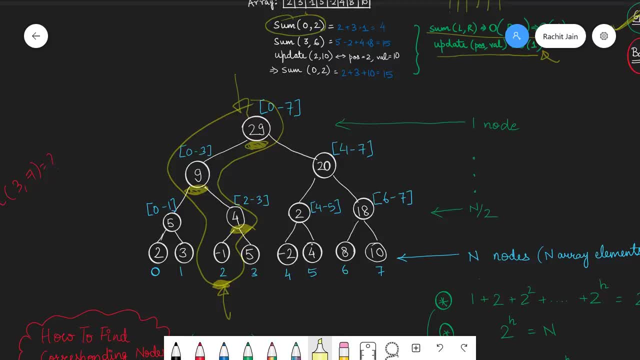 we update 2 to 10. essentially, what is happening is that we are getting a set of nodes which are falling in the path from all the way from the root to the leaf node which is changing, So in the complete tree we only have a particular set of nodes which are changing and that's nothing but the nodes which are 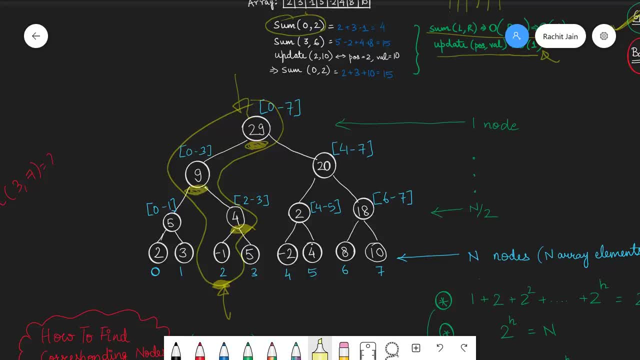 falling in the path from all the way from the root to the leaf node, which is changing. So when we update 2 to 10, essentially what is happening is that all the nodes in this path will get incremented by a value 11, because this leaf node is changing from minus 1 to 10. it's a